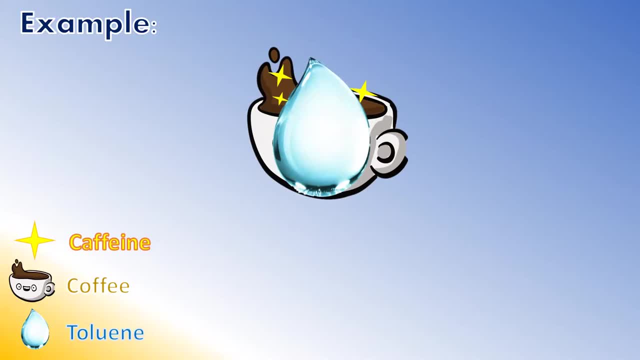 the prince and the sparkles with the caffeine is act like the princess, and in this case we take that as snow white. So this cup of coffee is like the evil witch: The snow white could be saved by the prince with the hands of the evil witch. This means that the caffeine 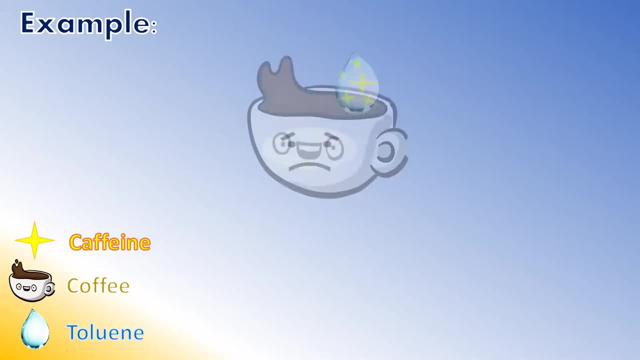 are being pulled out from the coffee into the toluene And, after the extraction caffeine, the mixed coffee will start to form two layers. so what? the upper layer is the toluene with the caffeine, while the lower layer is left with the coffee with much water in it. 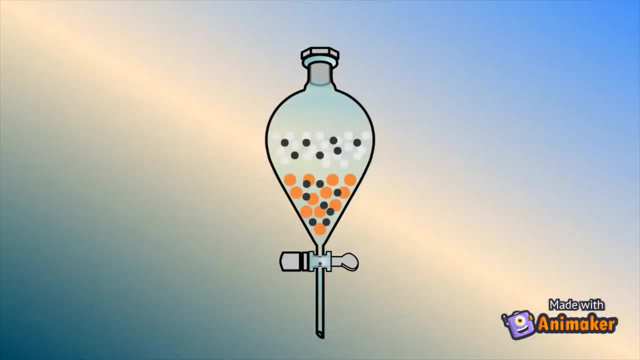 your toluene is to be mixed with coffee. in this case, toluene is like a prince, caffeine is like snow white and water is like the evil witch during the missing. we want the prince to rescue the snow white from the evil witch. this means that caffeine is being pulled out of the coffee into the toluene. 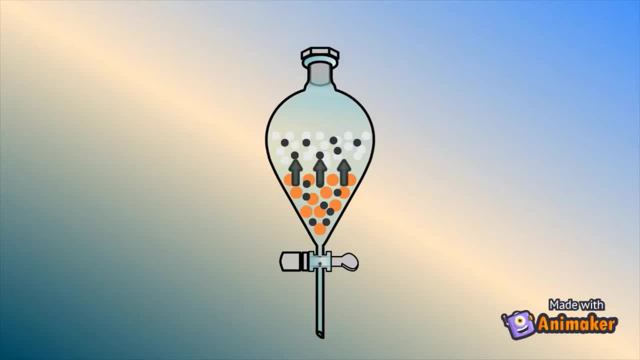 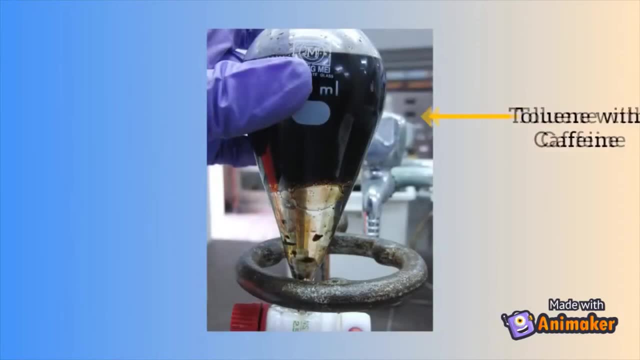 we can say that the caffeine is being rescued by the toluene. after the extraction of caffeine, the mixed coffee, after a while will start to form two layer. the upper layer is the toluene with the caffeine, while the lower layer is the left coffee which with much water in it. 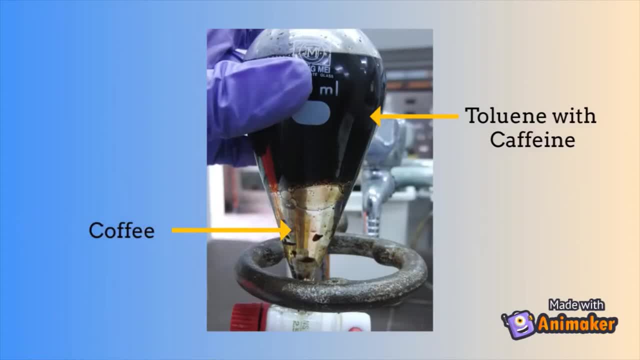 so you might wonder that why does this happen? this is because caffeine is toluene and water is toluene. so you might wonder that why does this happen? toluene and toluene, both is organic, while the water is inorganic. caffeine has higher solubility. 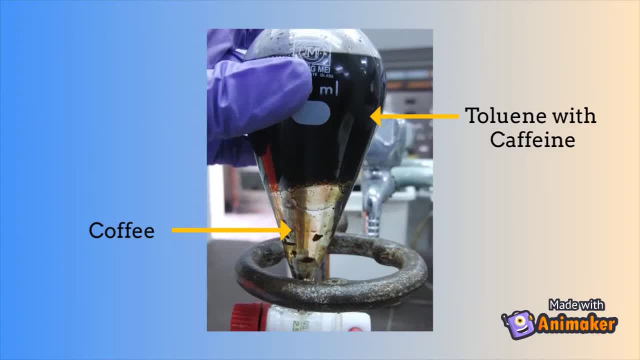 in toluene than it is in water. because of this, when the coffee is mixed with the solvent toluene, the toluene molecule will extract the caffeine molecule from the coffee. the caffeine molecule is absorbed into the toluene molecule and form the upper layer. 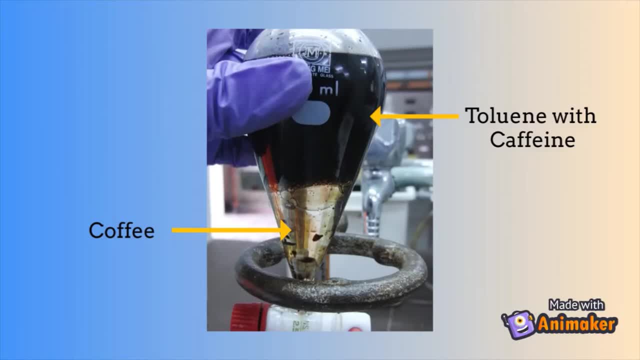 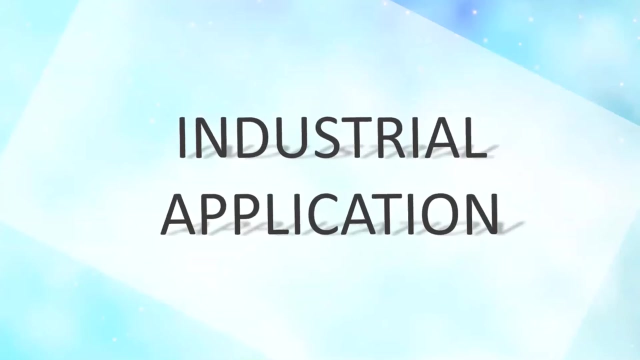 due to toluene has lower density than water, so the toluene will float on the top of the water. hence the two-layer system will form. to perform this same action on an industrial setting, we need to make sure everything can be carried out in large still and continuous. 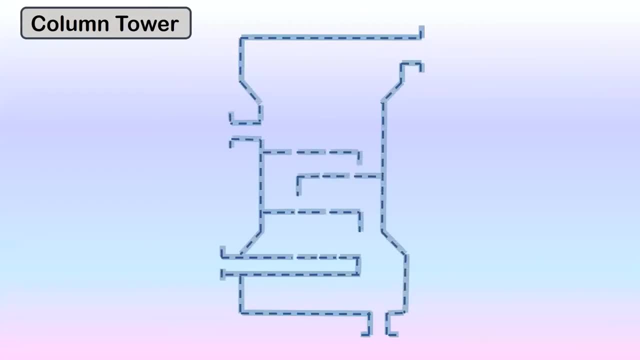 to do this we will need a specific equipment such as this column tower. to begin, the coffee will first fill in the column, then toluene will spray from an entrance just above the bottom of the column. to begin, the coffee will first fill in the column, then toluene will spray from an entrance just above the bottom of the column. 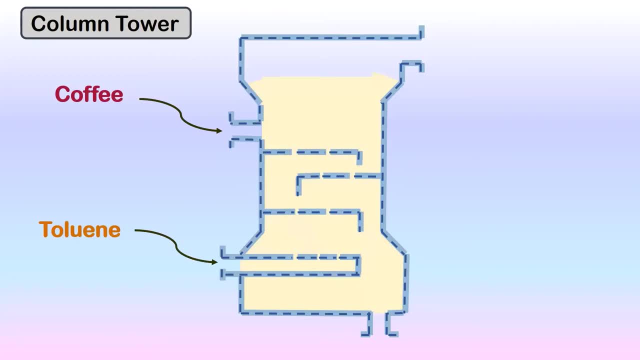 the column into the coffee. The density difference will make the toluene flow upward. When the toluene flowing upwards, the interaction between coffee and toluene will transfer the caffeine from coffee into the toluene, The toluene which now contains the caffeine. 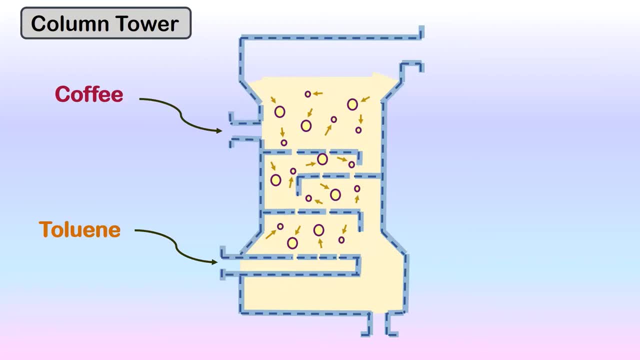 continue to move upwards until they eventually settle as a new layer on top of coffee. The coffee that has its caffeine removed will be found at the bottom of the column, where it will eventually be expelled out. The toluene-carrying caffeine will then exit from above. 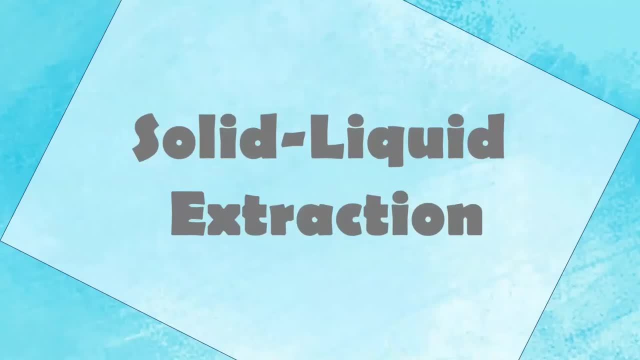 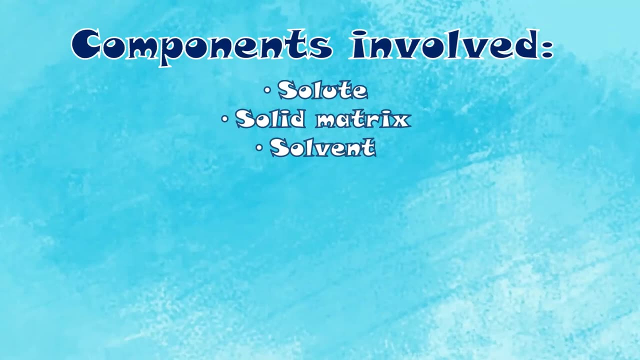 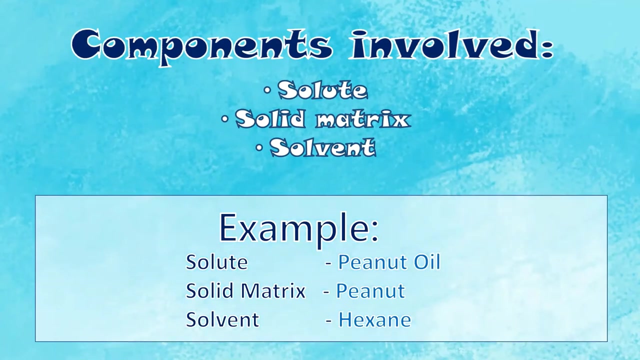 Next, we are going to talk about solid-liquid extraction. The components involved in solid-liquid extraction are solute, solumetrics and solvents. Today, we are going to take the extraction of peanut oil from peanut using hexane as an example. 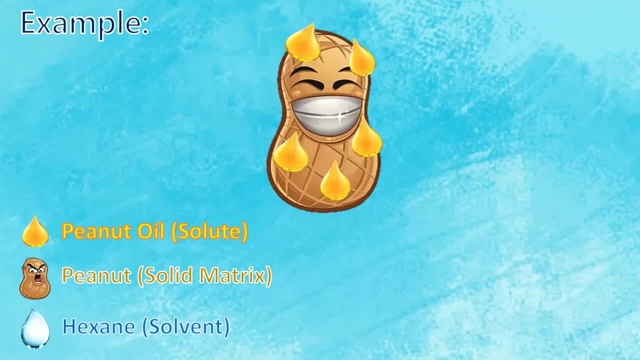 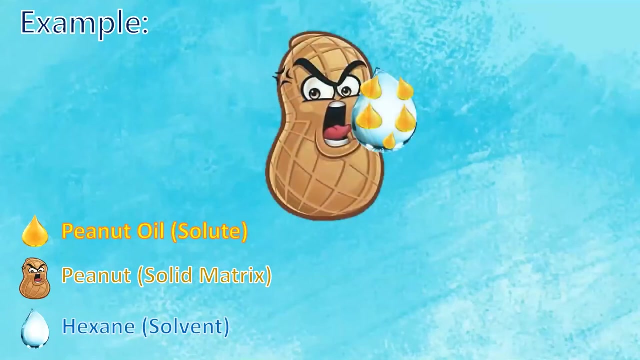 Solute. the component to be extracted from the solid matrix is peanut oil. while peanut will be our solid matrix, Hexane will be used as our solvent. The operating extractor is divided into two layers: lower layer and upper layer. The input of the 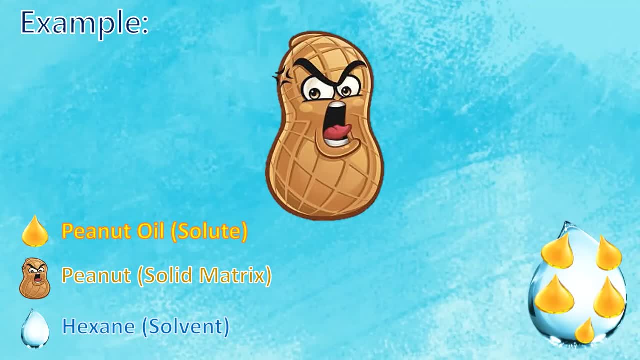 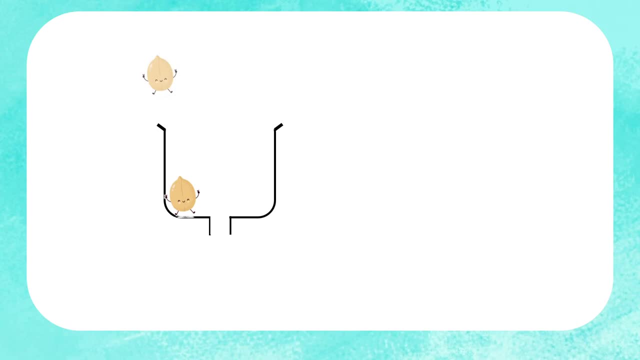 lower layer will contain solid and solute, while the input of the upper layer will contain only solvent. Firstly, we have our solid peanut containing solute peanut oil entering the lower layer. In this figure, peanut oil is represented by the hands and legs of the peanut, Then hexane. 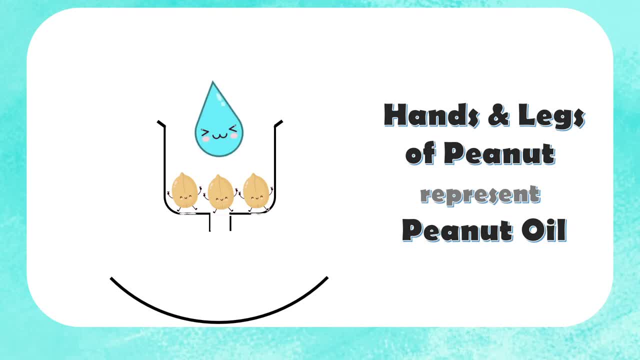 which is a solvent, is entering the upper layer. Upon contacting, the extraction process takes a place. Peanut oil will be transferred from solid peanut into hexane. This is because peanut oil has higher solubility in hexane. Peanut oil is more comfortable when staying with hexane.